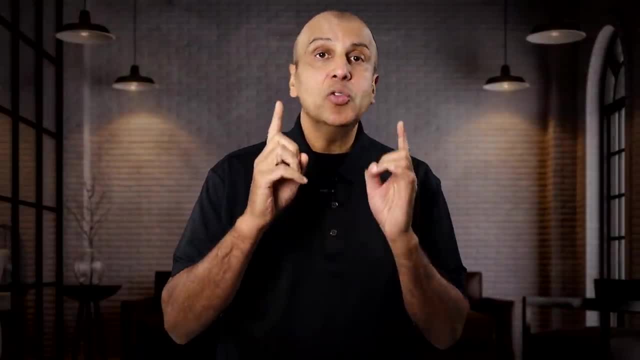 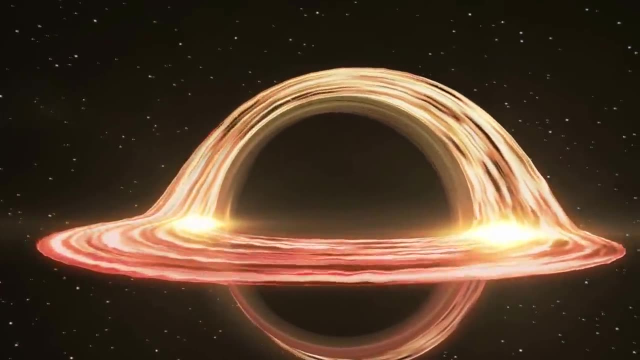 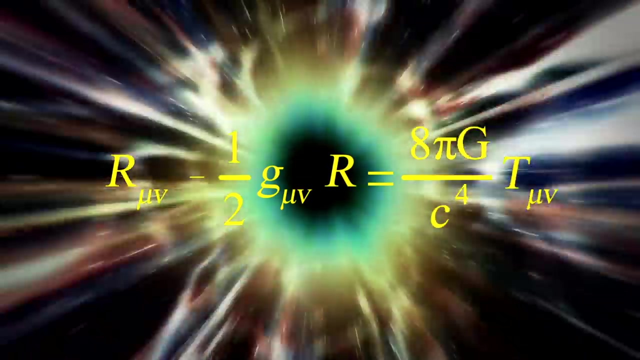 Is it also at multiple locations at the same time? There is no such thing as superposition in general relativity. Another problem occurs in the case of black holes. There is a region of space called the singularity, where matter and energy is supposedly compressed to an infinitely small point, with 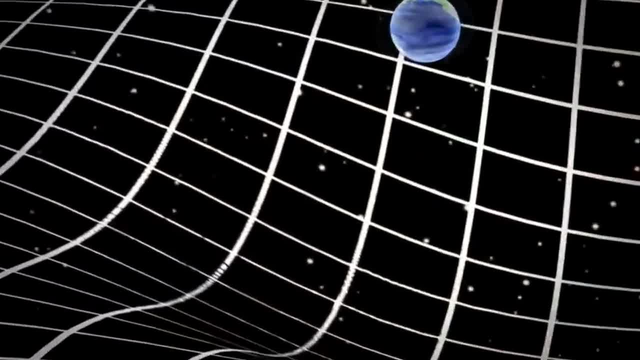 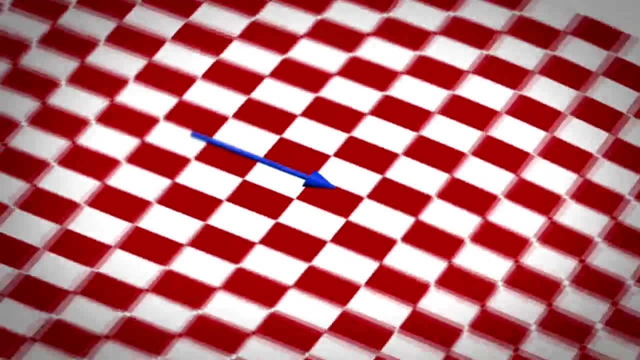 infinite curvature of spacetime. But the equations of general relativity treat spacetime mathematically as being flat at infinitesimally small distances and then calculate the overall curvature based on this presumption. This does not work at the singularity, because infinite 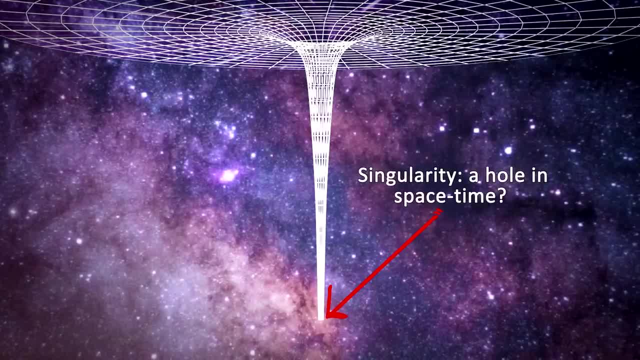 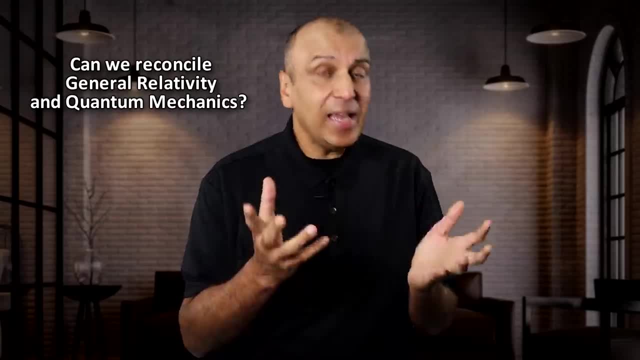 curvature at an infinitesimally small distance is not the same as the curvature at an infinitesimally small point, results in nonsense, results in the math of general relativity. So the question is: is there any way we can reconcile these two highly proven theories? 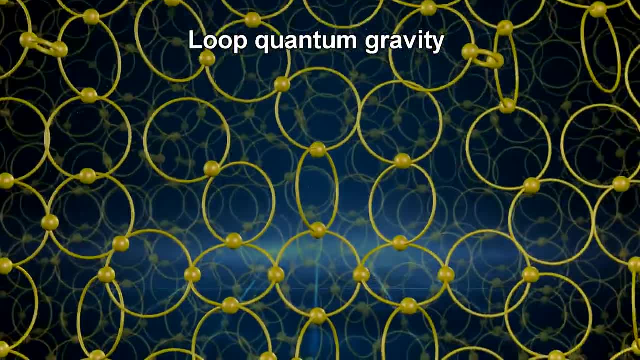 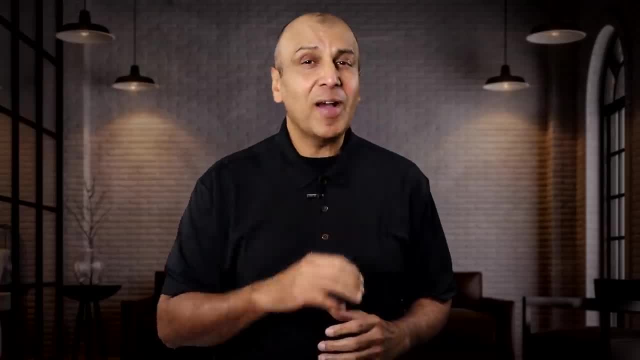 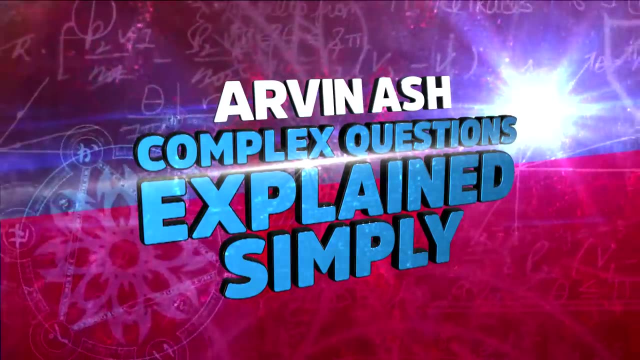 so that we can have a true picture of how reality works. Well, there are two theories that attempt to tackle this reconciliation: loop, quantum gravity and string theory. The explanation of how these two theories work is coming up right now. Before I get into loop, quantum gravity and string theory, let me tell you what inspired 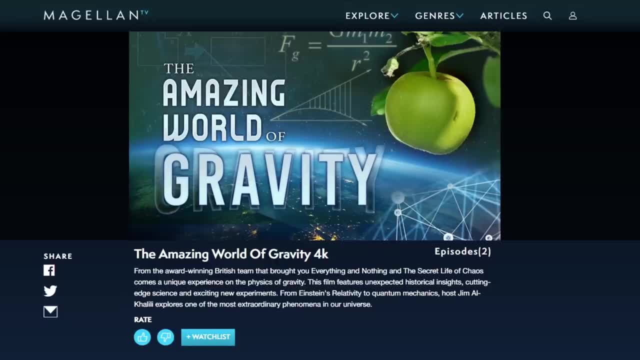 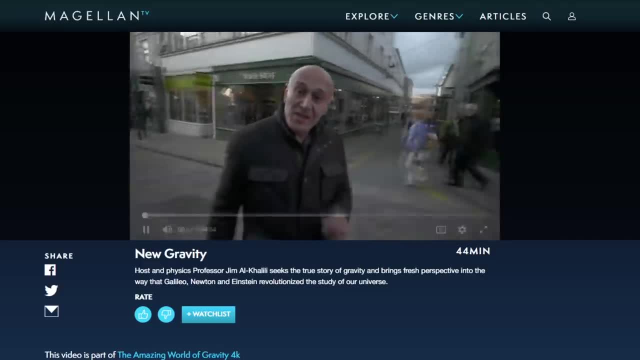 me to do this video. I recently watched a two-episode documentary on Magellan TV, today's sponsor, called The Amazing World of Gravity. It's hosted by one of my favorite educators, Jim Al-Khalili, and it's in 4K. Magellan is a new type of streaming documentary service. 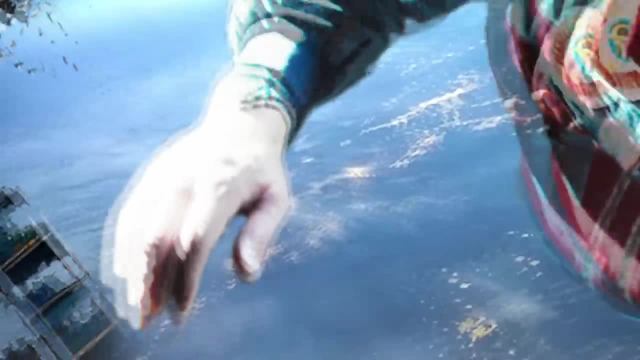 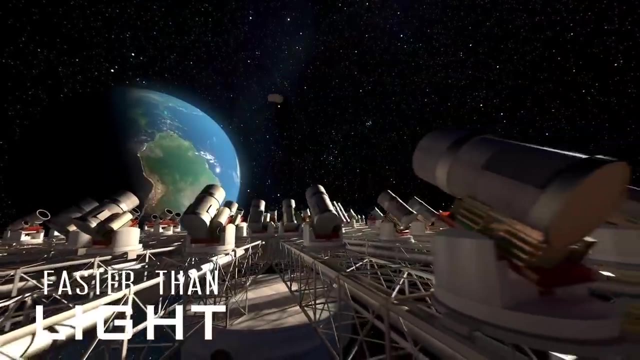 founded by filmmakers and producers who bring you great, premium documentary content. Featured subjects include history, nature and- my favorites- science and space. Magellan TV is a great source of information. You can watch it on any of your devices, as well as your TV anytime. 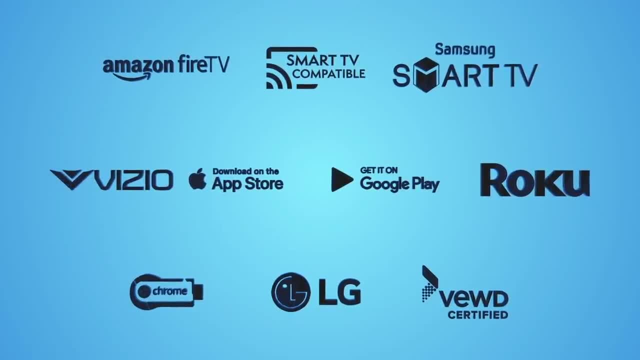 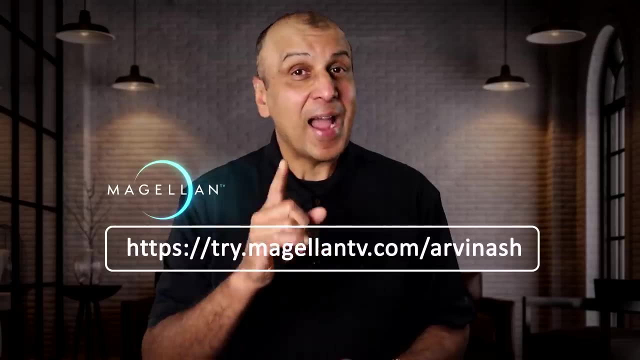 without any ads and they have a huge library of 4K content. Magellan TV has a special offer right now for Alvin Ash viewers. If you use the link in the description, you'll get a free one-month trial. I highly recommend Magellan TV, but be sure to use the link in. 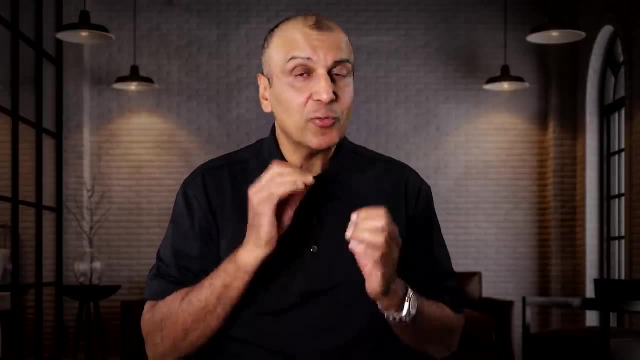 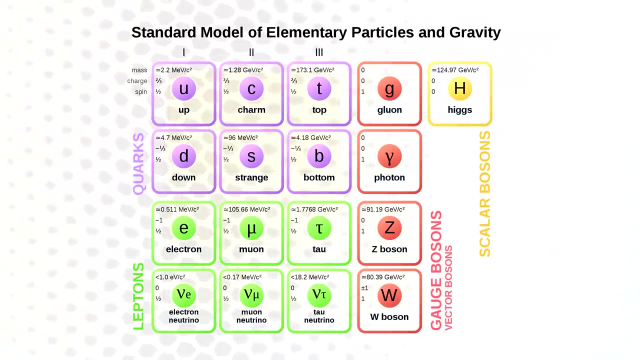 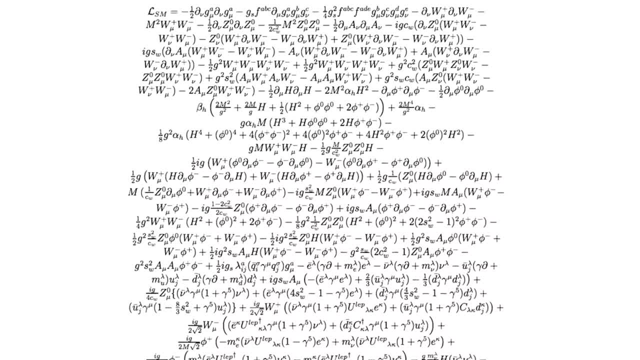 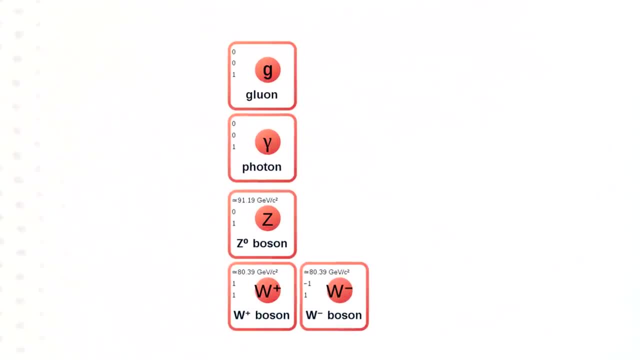 It is really a visual representation of many equations that are behind it. Here's a glimpse of what those equations look like. I want to draw your attention to the red-gauge bosons on the chart. These represent the fundamental particles responsible for three of the four. 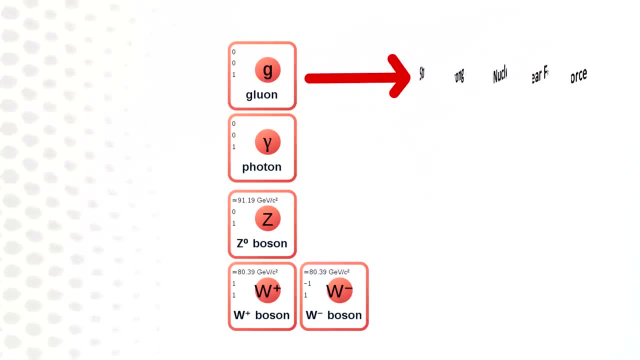 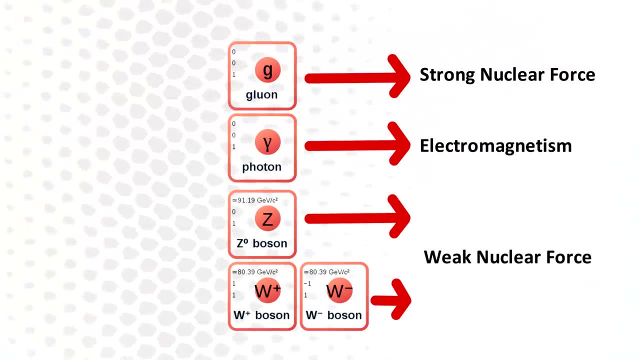 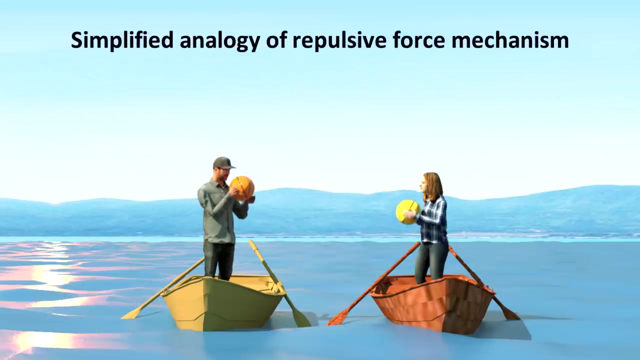 known forces in the universe. The gluon is responsible for the strong force, the photon is responsible for electromagnetism and the W and Z bosons are responsible for the weak nuclear force. The way a force is conferred is through the exchange of virtual bosons. So, for example, in electromagnetism, an exchange of virtual photons results in. 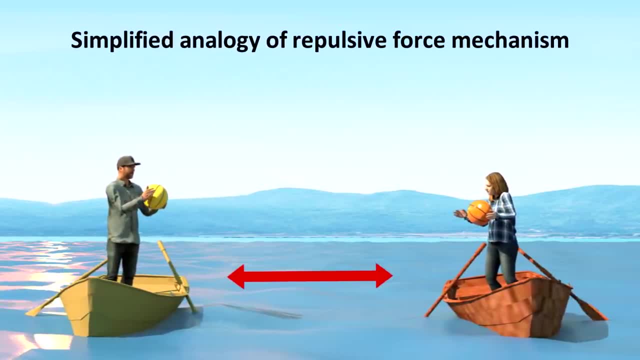 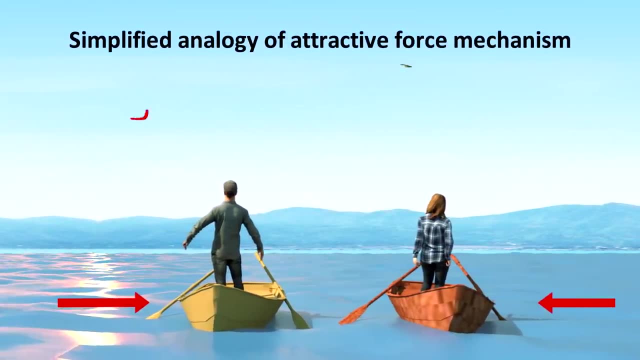 an exchange of momentum which results in two like charges repelling each other. Attraction happens through the exchange of negative momentum, similar to this boomerang analogy. I made a video recently on how these forces work at the subatomic level, if you are interested. 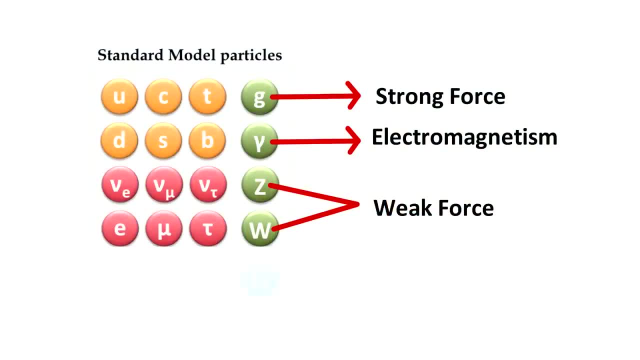 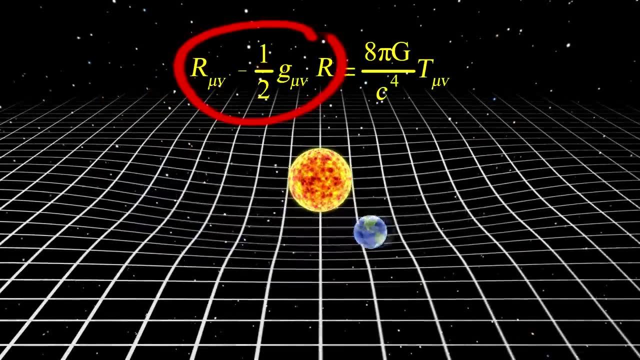 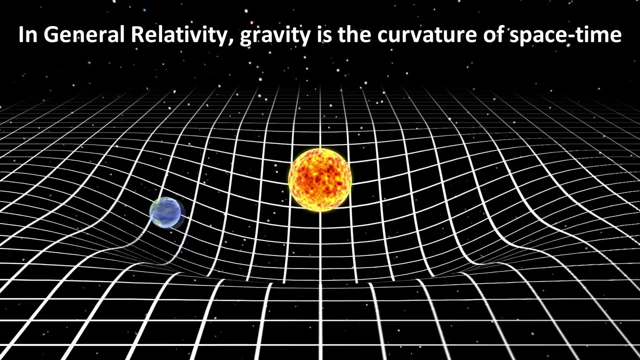 in viewing it, You'll notice that one force is conspicuously missing from this picture, and that is gravity. This is because, according to our best model for gravity, Einstein's general relativity, gravity is not a force, but is a result of the curvature of the background. 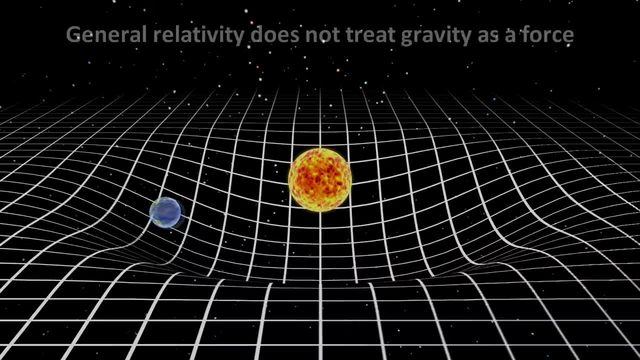 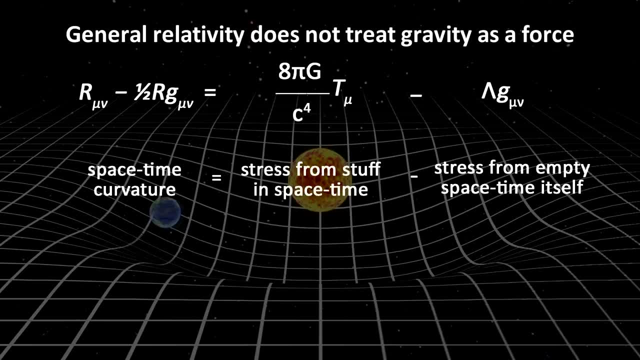 the curvature of space-time. But the equations of general relativity treat space-time as a bending of the continuous background of space-time, not as a result of discrete particles that confer a force. This is a problem. Stars and planets are made of molecules, atoms. 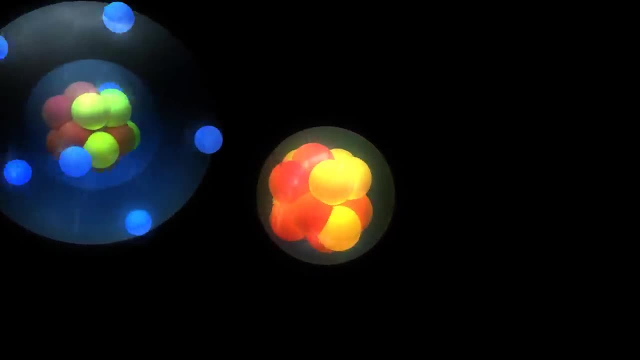 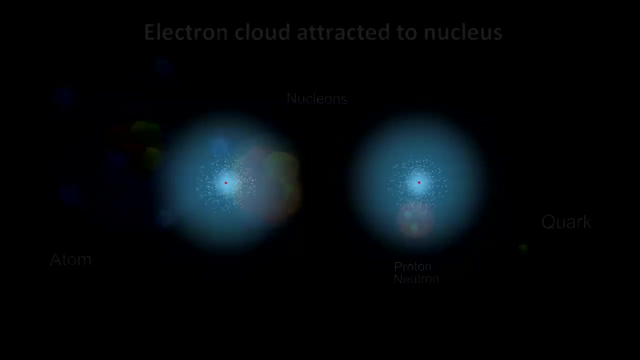 and radiation. These are ultimately made up of elementary particles of the standard model, And we know that these are made up of discrete units of energy, And the forces that hold the atoms together are also due to discrete units of virtual particles represented by the gauge. 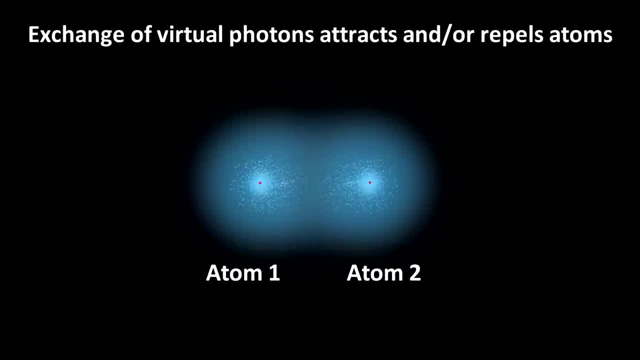 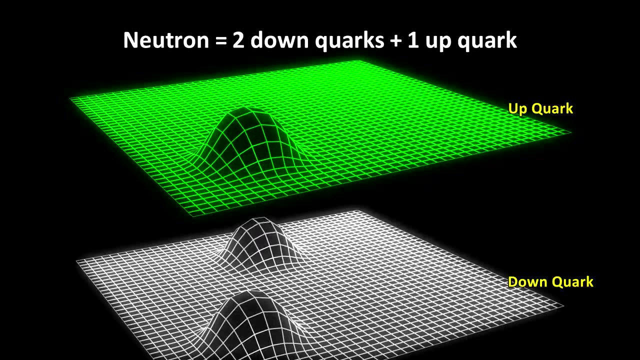 bosons, And it's the exchange or swapping of these virtual bosons that holds and breaks up atoms and molecules. The universe is bumpy. There is no such thing as continuous matter and energy. This is why Einstein's general relativity is so important. This is why Einstein's general 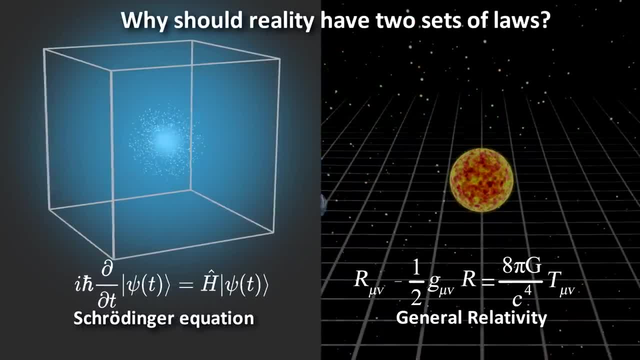 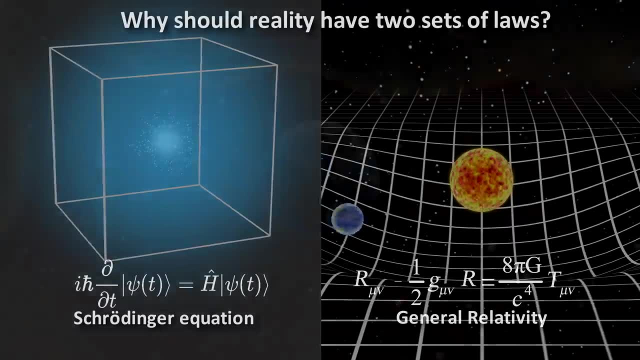 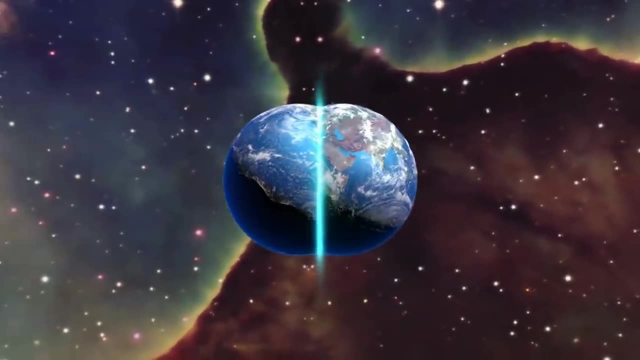 relativity is so complex, Why should reality have two sets of rules: Quantum mechanics very small and general relativity very large. Even if they appear to follow two separate rules, they should unite at some fundamental level. One set of laws should emerge from. 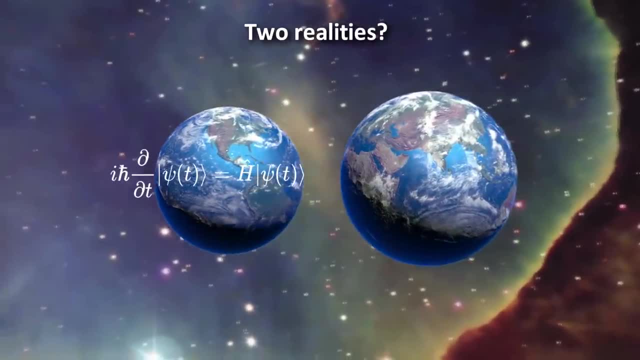 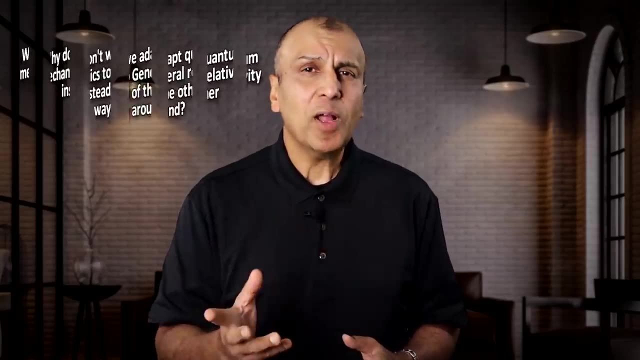 the other, because we live in one reality, not two different realities. This is partly the reason that most physicists believe general relativity is incomplete. You could ask well why. If you want to know why, pause this video. You'll come to the 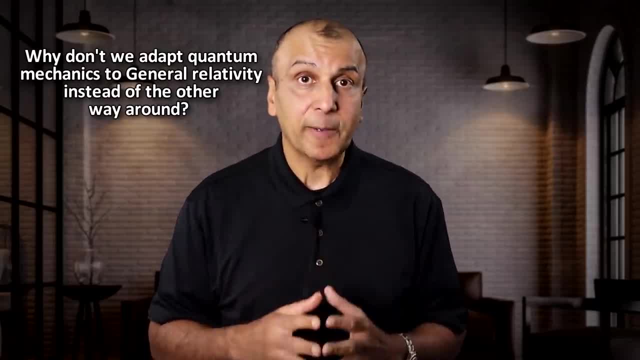 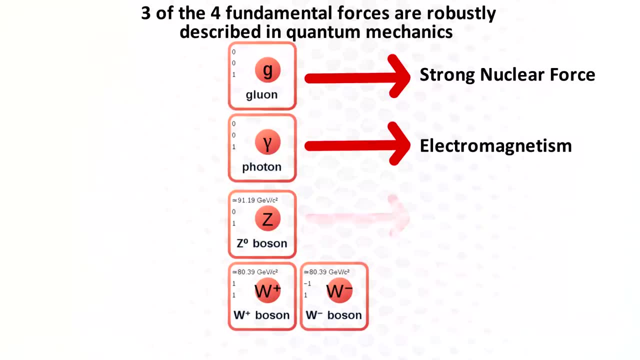 following slide. can't quantum mechanics be the one that is incomplete? Here's part of the reason. Of the four fundamental forces, three have very robust theories rooted in quantum mechanics. Only gravity lacks a quantum description, Not only the forces, but also the vast majority. 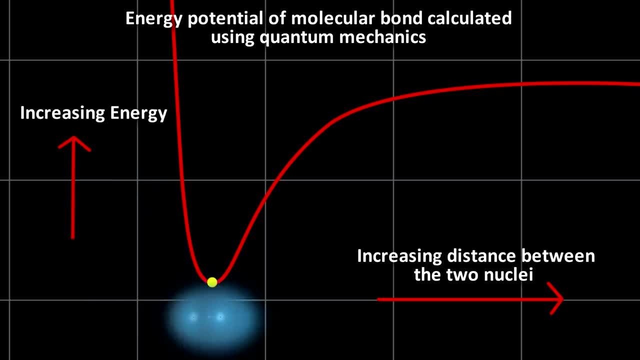 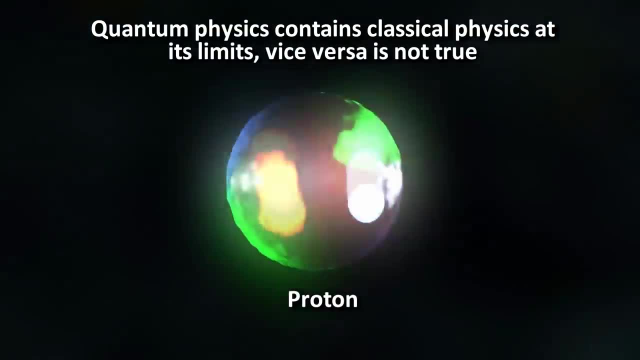 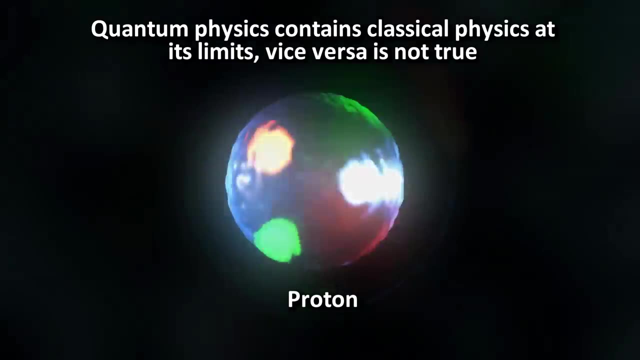 of particles, including atoms and molecules, have very robust quantum theories explaining them. Quantum mechanics also has almost all of the classical physics within its limits. On the other hand, classical physics, like that of general relativity, does not include any quantum effects. We came up with quantum theories because classical physics did not. 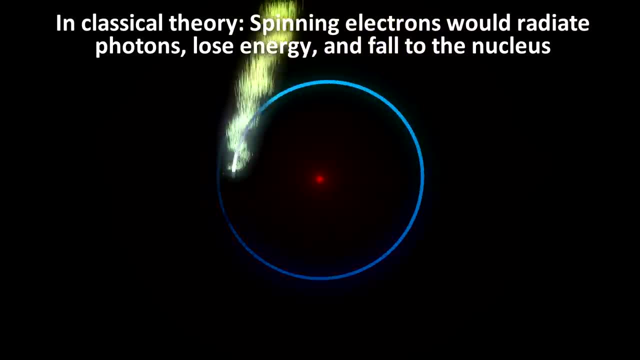 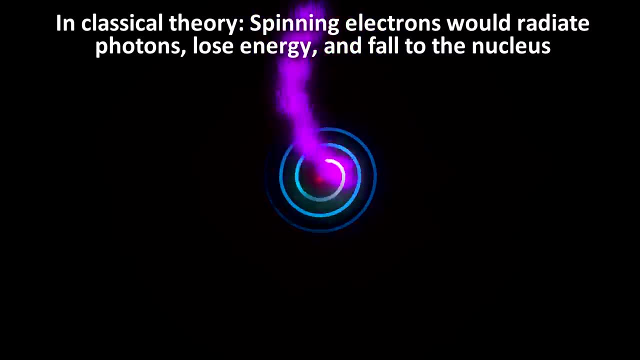 work under all circumstances, and it could explain more observations. What we've learned in the past 90 years is that quantum physics is the fundamental language of reality. This is why it is thought that gravity needs to be brought into the fold and not the other. 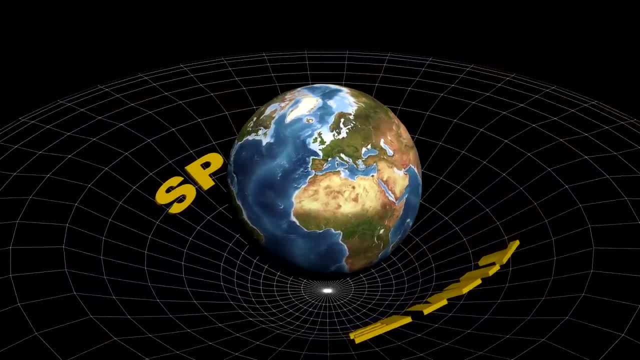 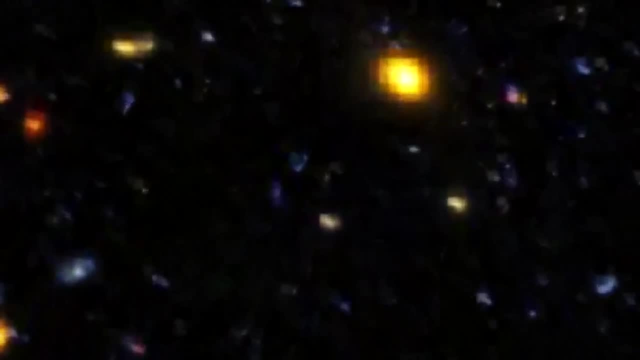 way around. Now, one way to do this is to hypothesize. We hypothesize that perhaps the background, space-time itself is quantized. This is what loop quantum gravity, or LQG, attempts to do. It attempts to show that the fabric of 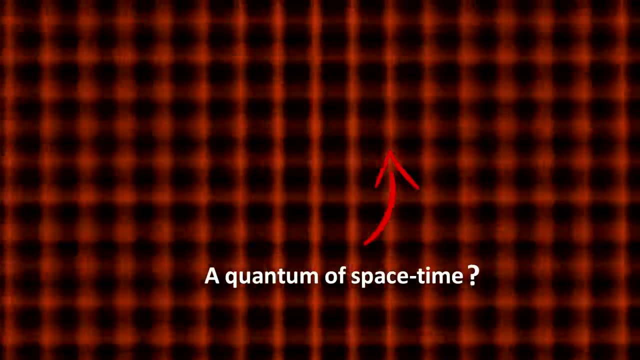 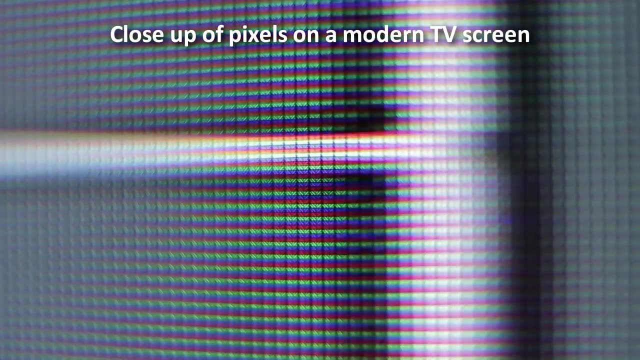 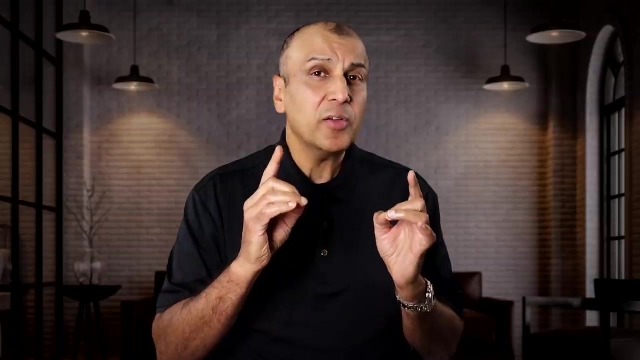 space-time is not continuous, as Einstein presumed, but is itself made up of discrete quanta. Think of a TV screen. Even an HDTV, at its smallest level, is made up of discrete pixels which cannot be further reduced. This is different from every other theory, including 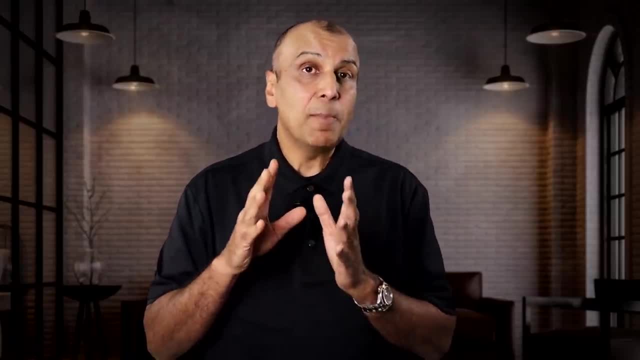 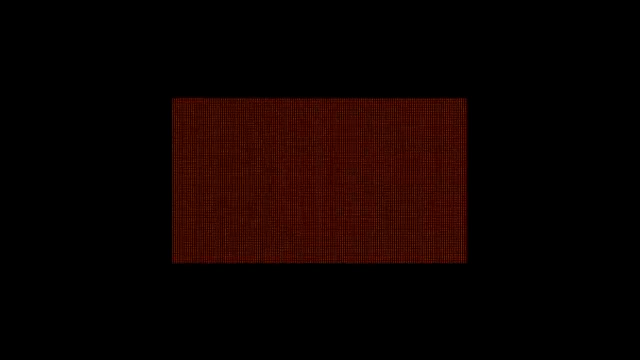 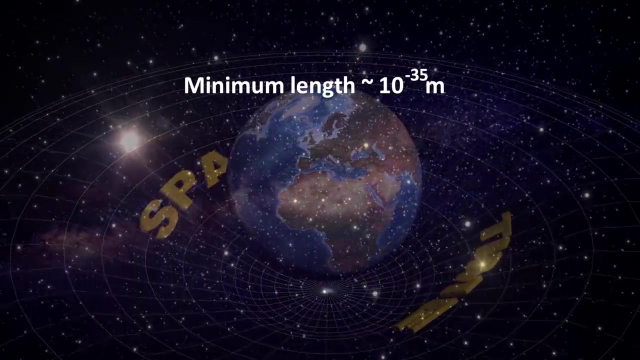 string theory, Because even in string theory space is the background or canvas on which strings vibrate. In LQG this space-time background is itself quantized, like your television. So this means that distance has a minimum quantity about equivalent to the Planck length, or 10 to. 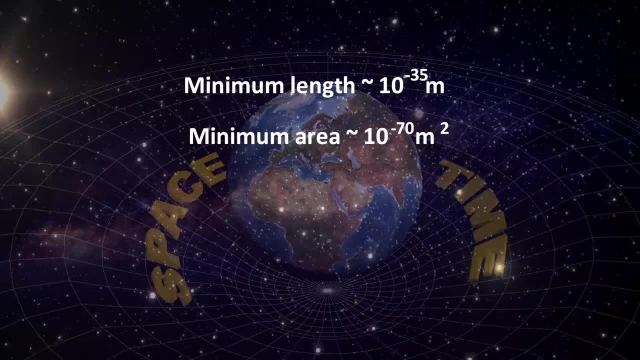 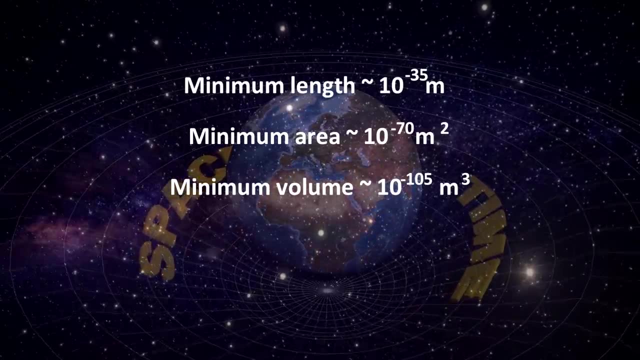 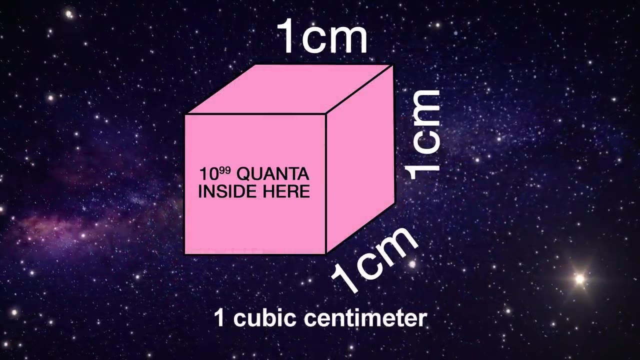 the negative 35 meters. Similarly, area has a minimum value of 10 to the negative 70 meters squared and volume has a minimum value of around 10 to the negative 105 meters cubed, below which it cannot go. This is super tiny, To give you an idea of the smallness of the scales we're talking. 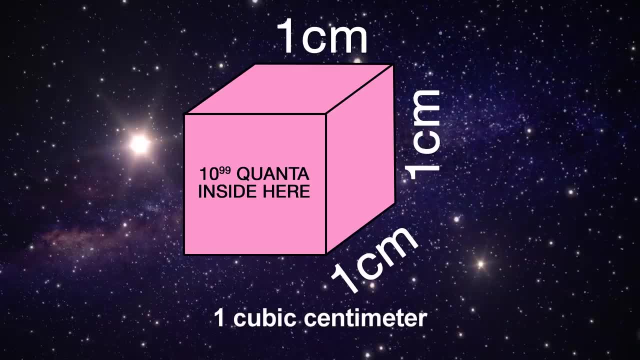 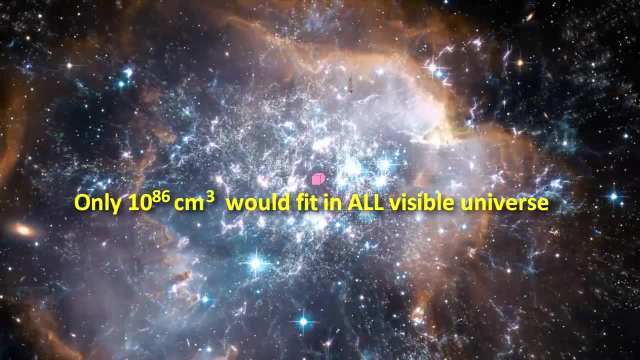 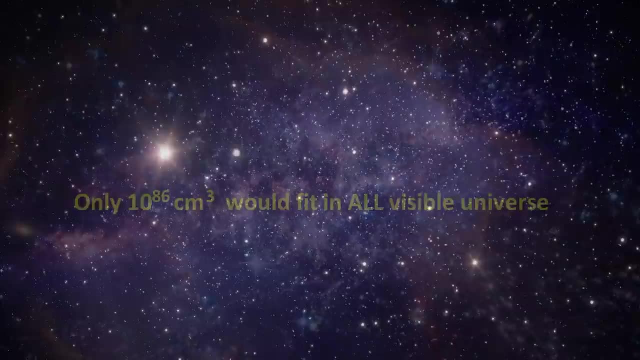 about. LQG says that there are about 10 to the 99 quanta of volume in every cubic centimeter of space. This quantum of volume is so tiny that there are more such quanta in a cubic centimeter than there are cubic centimeters in the entire visible universe And time itself. 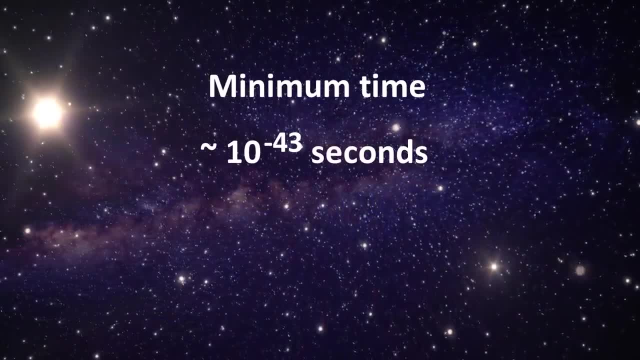 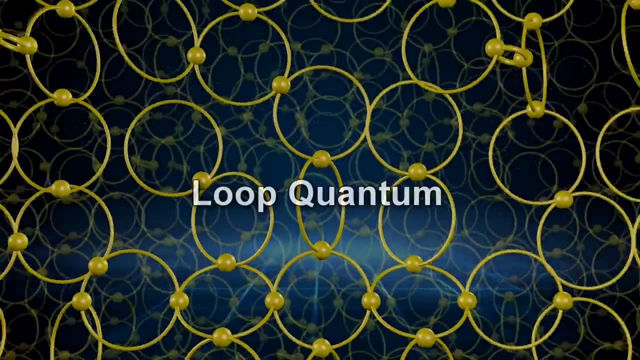 has a minimum quantity as well, which is about 10 to the negative 90 meters. This is super tiny, but it's not a big deal. And what do these space-time quanta look like? Well, space-time is basically made up of finite. 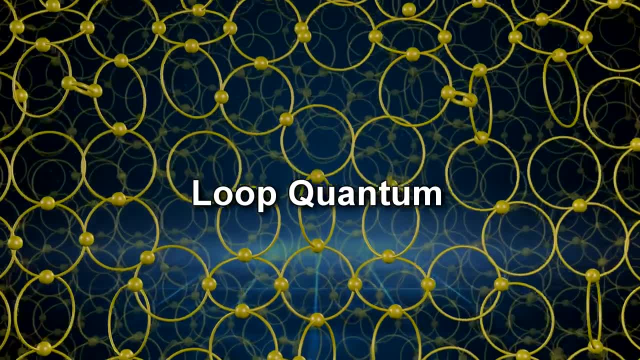 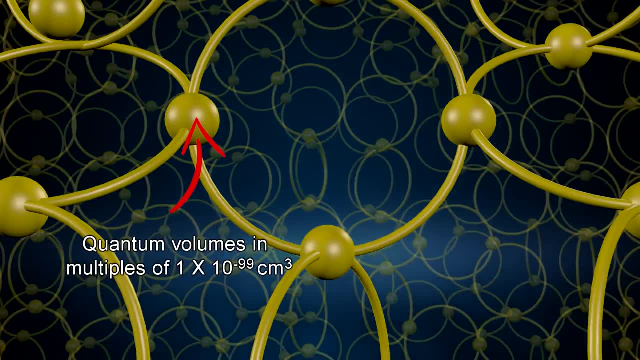 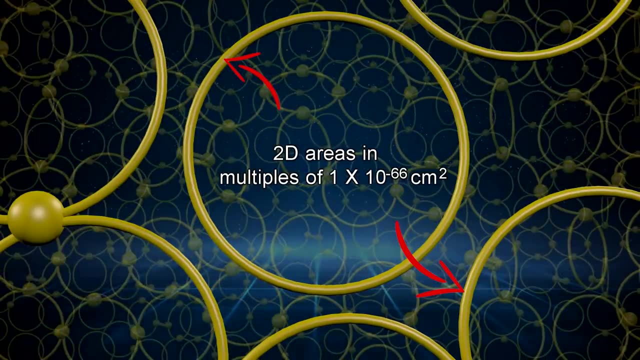 loops with nodes connecting them. The nodes that intersect is where the quanta volume of space reside. It has a volume that is a multiple of the Planck volume 10 to the negative 99 cubic centimeters. The loops in between these nodes represent two-dimensional areas. And large quantities of these loops are connected to each other. So the quanta volume of the space-time quanta is a multiple of the Planck volume 10 to the negative 99 cubic centimeters. The loops in between these nodes represent two-dimensional areas And large quantities of these loops. 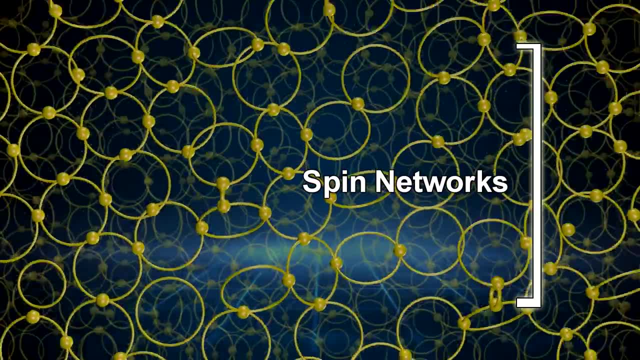 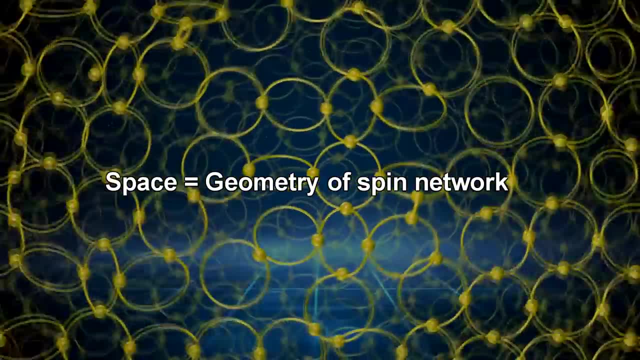 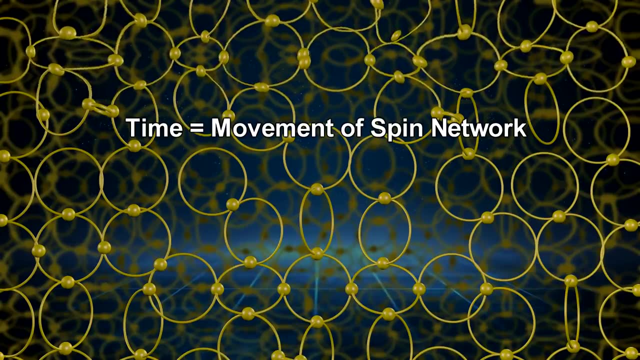 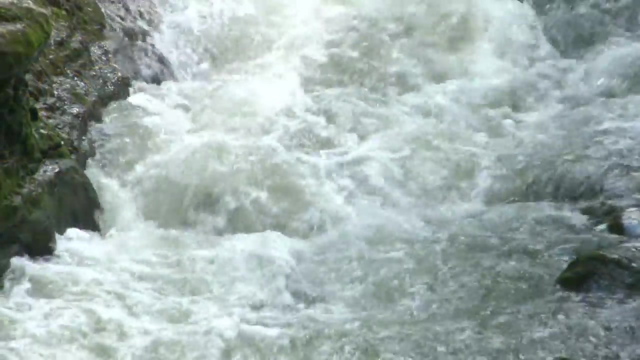 and nodes are called spin networks because their properties are related to a particle quality called spin. Space is defined by the geometry of the spin network, and time is defined by the moves that rearrange the spin network. The spin network, when combined with these quantum movements of time, is called a spin foam. Time does not flow like a river In. 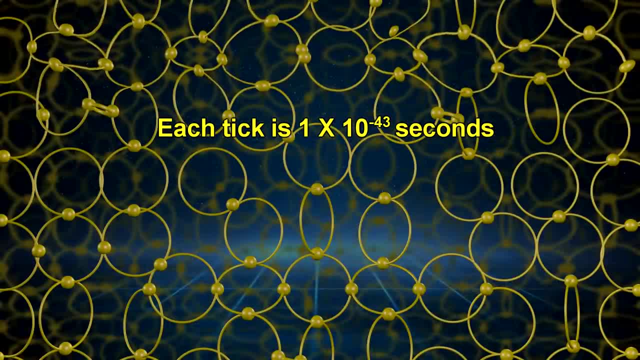 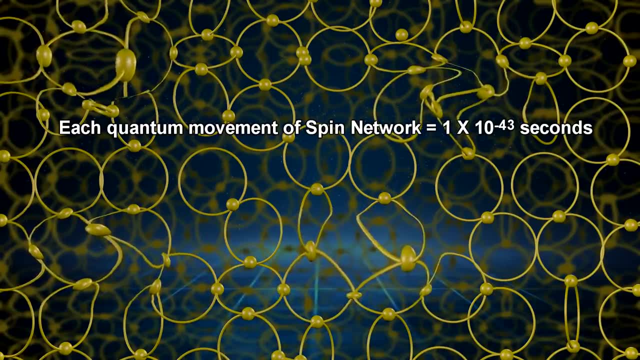 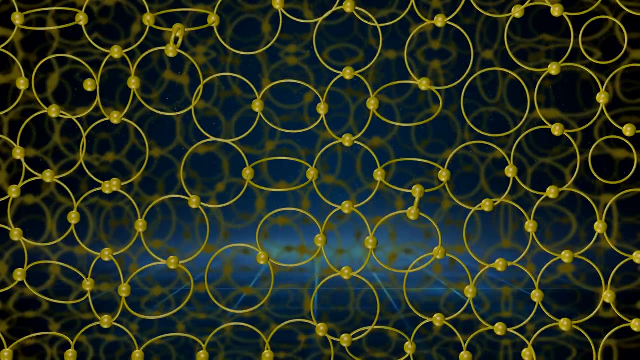 the spin foam. it ticks like a digital clock And each quantum tick or movement is called 10 to the negative 43 seconds. Every location in the spin network where a quantum move takes place, time has ticked once. How do particles traverse this quanta space When mass and 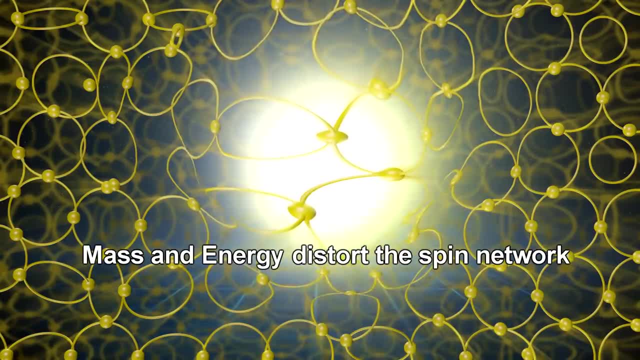 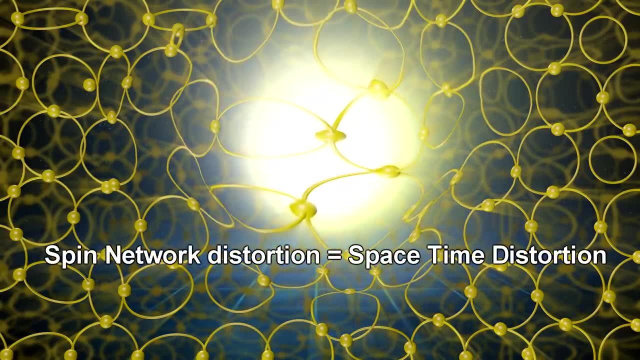 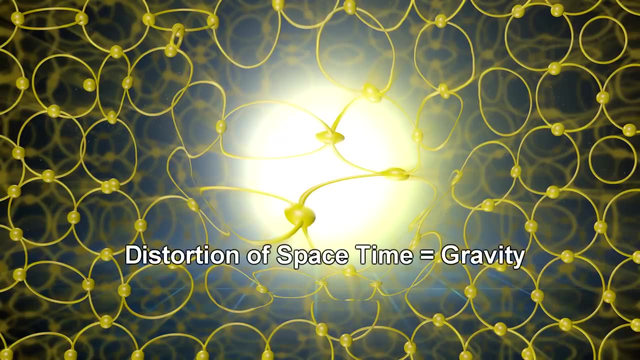 energy are added to the spin foam, the shape of the volumes of the spin network is distorted. This distorts space and time, because any movement of these quanta also affects the time quanta. Time is essentially movement of these volume quanta And this distortion of space and time. 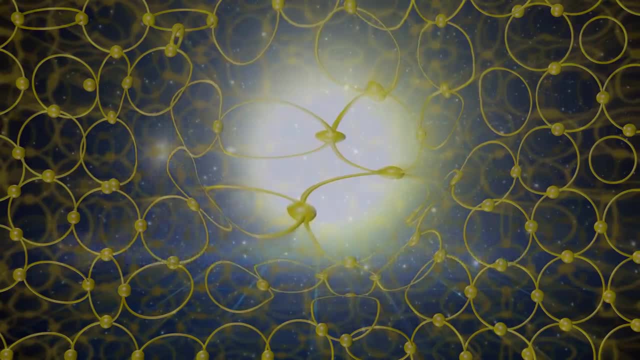 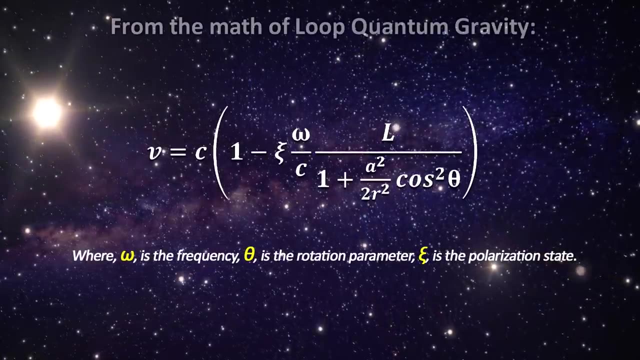 is what we perceive as gravity. The exciting thing about LQG is that it makes some predictions that could be tested. For example, it predicts that the speed of light has a small dependence on energy. Photons of high energy travel slightly slower than lower energy photons. The effect 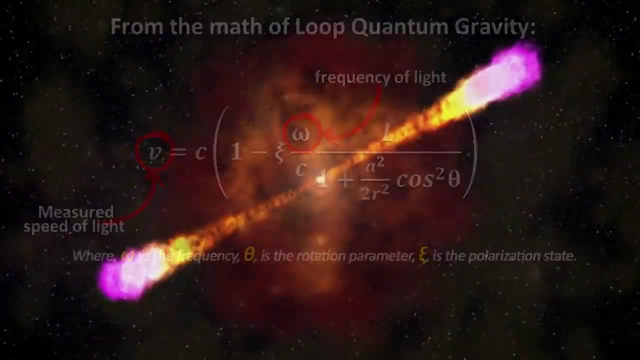 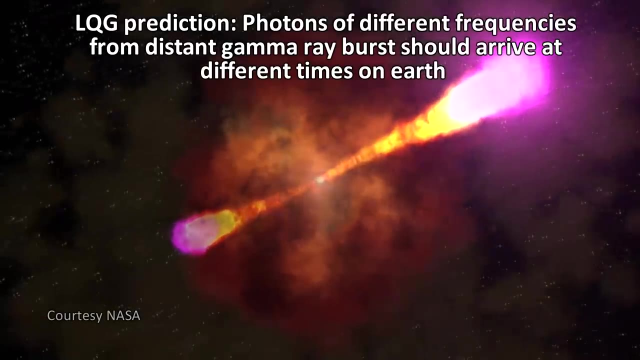 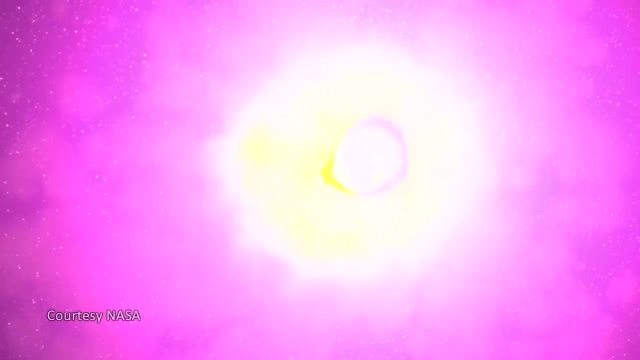 is very small but it amplifies over time. So two photons produced by a gamma ray burst, for example, billions of years ago, If they are of different frequency, should arrive on earth at slightly different times. And this time delay should be large enough to be detected by our instruments. But sadly, 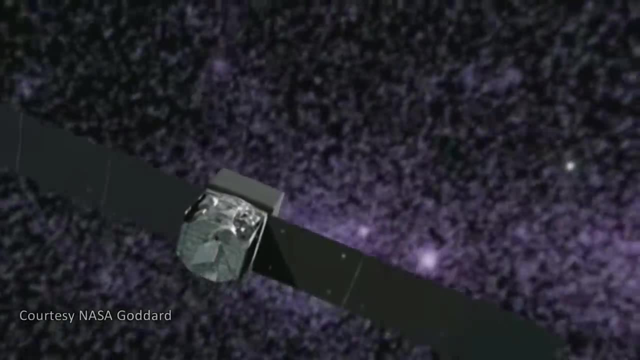 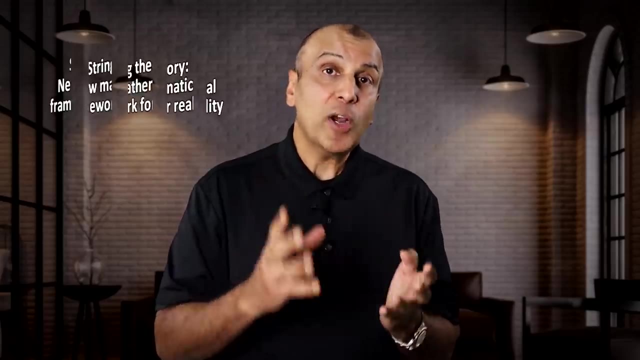 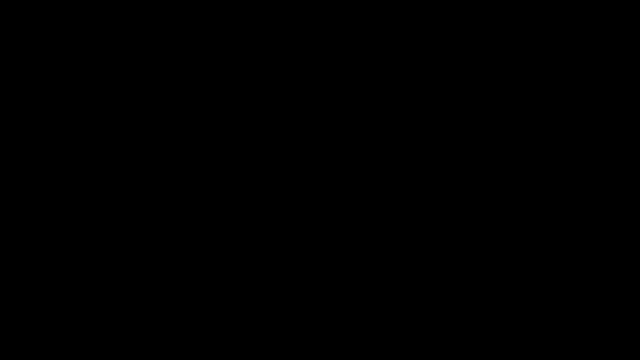 this has not been observed, It is possible that either the theory is wrong or our instruments are not sensitive enough. A second way to quantize gravity is to theorize a completely new framework of reality based on a new understanding of fundamental particles. This is what string theory attempts to do. 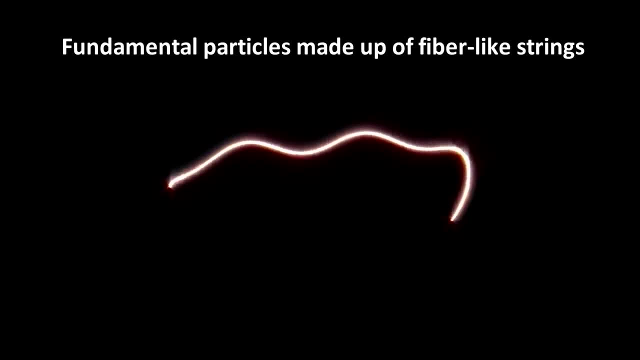 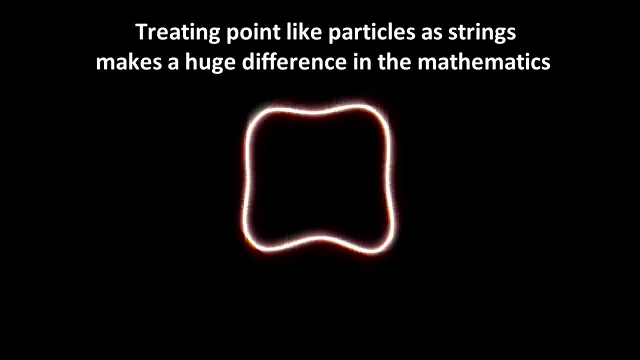 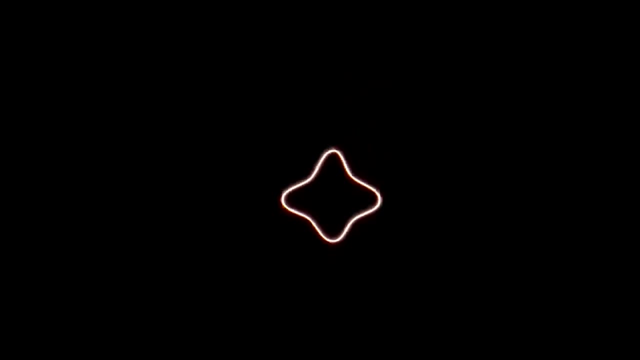 Basically, the fundamental particles of the standard model are replaced by something even more fundamental: One-dimensional fiber-like strings. The simple change of treating point-like particles as one-dimensional string-like particles makes a huge difference in the mathematics. If you take those strings and show that they can vibrate, it turns out that different types 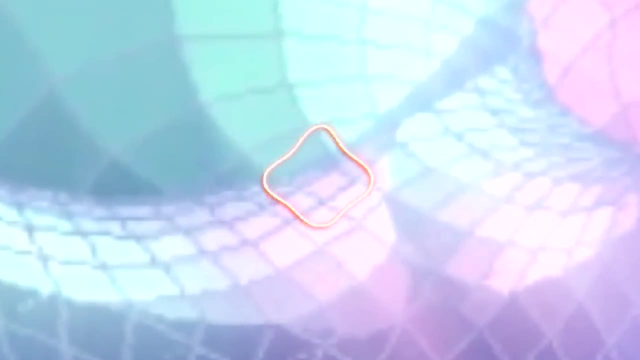 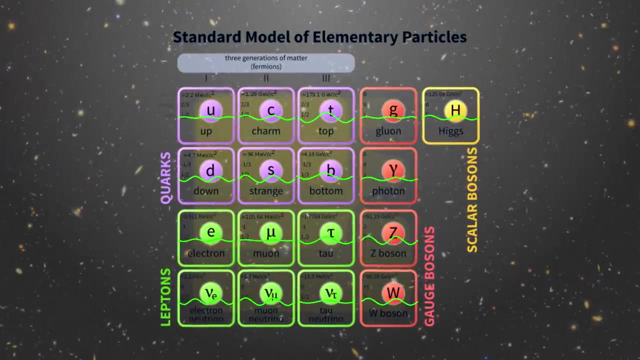 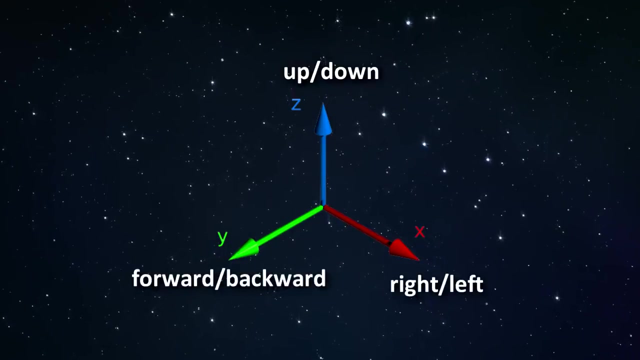 of strings with different vibrations behave just like the elementary particles of the standard model. So the various particles of the standard model can now be simplified by fundamental strings. This sounds great, but one of the biggest problems is that these strings would need to vibrate not just in the three spatial dimensions that we are used to, but in at least six more. 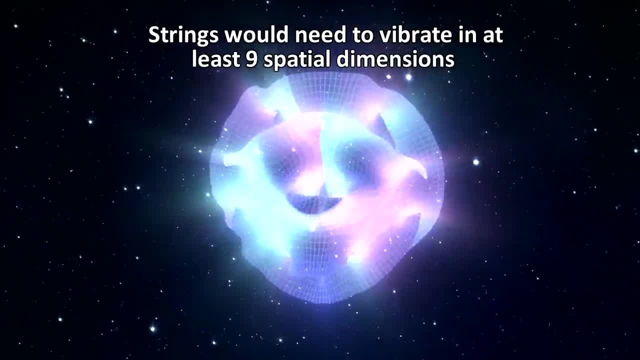 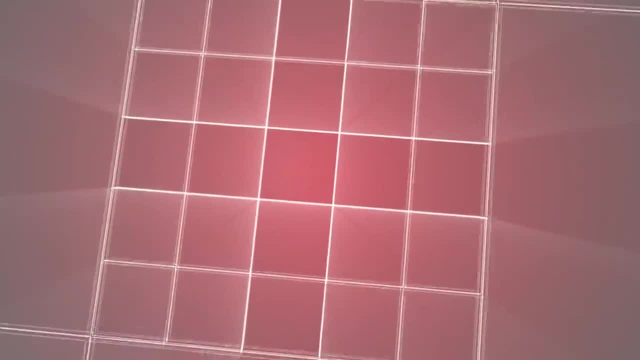 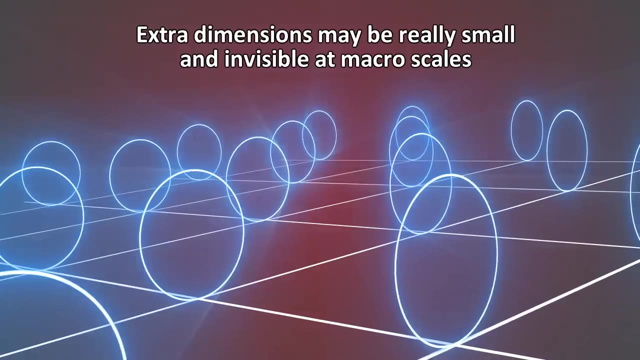 spatial dimensions in order to mathematically account for the various particles that we know of. So the question is: where are these extra dimensions? It does not appear that additional large dimensions in our universe exist, so physicists speculate. These dimensions could be very small and hidden from our perceptions. 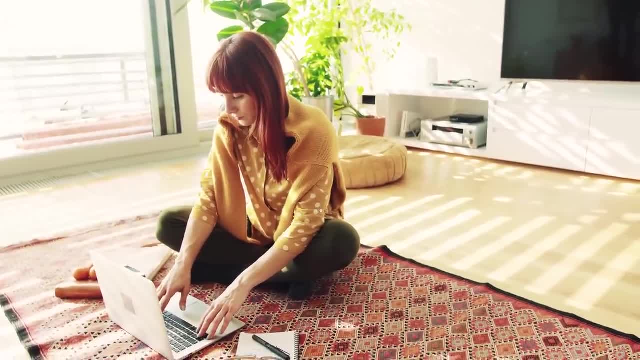 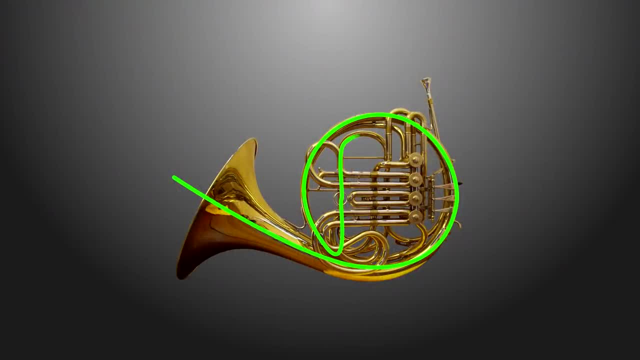 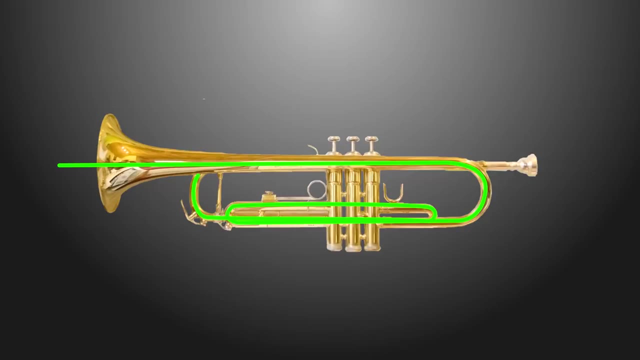 This is analogous to the way that a rug appears smooth from a distance, but if you look closely you'll see small loops and fibers in its structure. Strings vibrating in different dimensions is analogous to the way that a wind instrument can make different sounds depending on the way the air flows through its various surfaces. 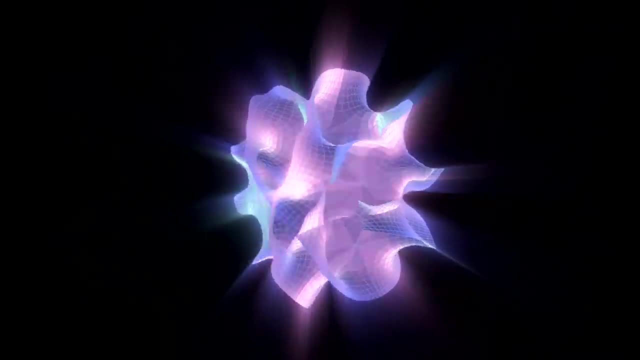 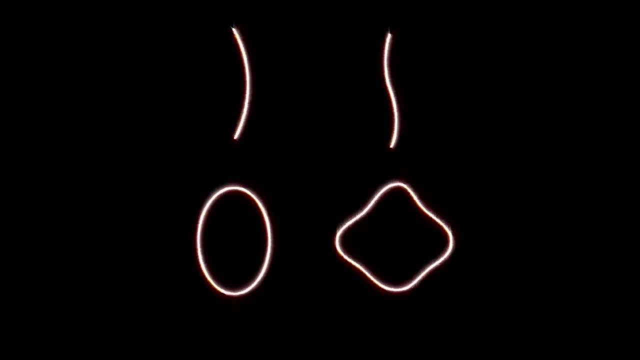 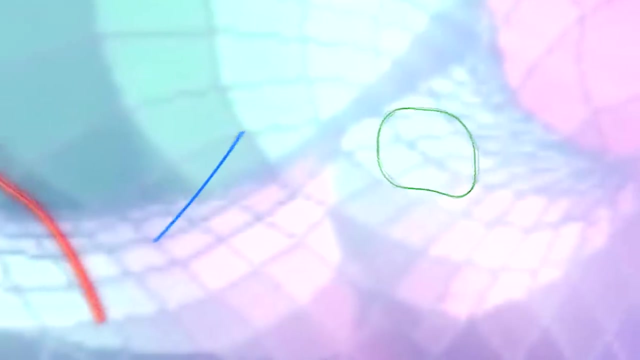 This is similar to the way that the same string can take on different properties when vibrating in different combinations of dimensions. These can be open strings or closed strings. The interesting thing is that if you treat the universe as strings vibrating in nine dimensions, a particular closed string vibration results in a unique graviton particle. 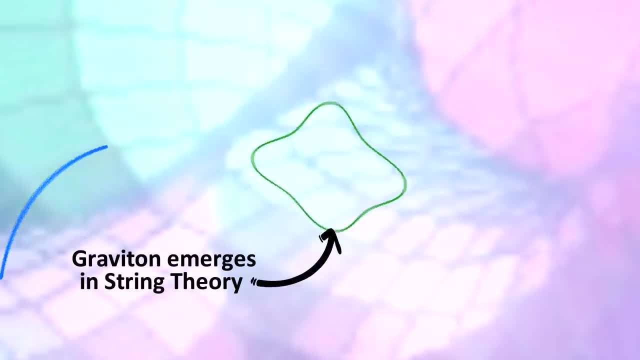 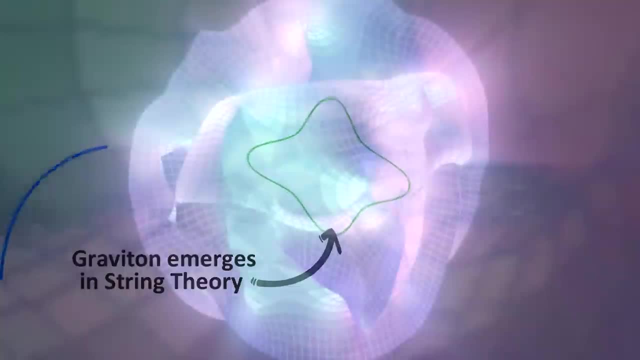 This appears naturally in the mathematics of string theory. so this would allow for the existence of a force carrying particle, just like the force carrying particles of the other three forces. Similarly, particular sets of strings and vibrations could account for the quarks, and particular vibrations could account for the quarks. 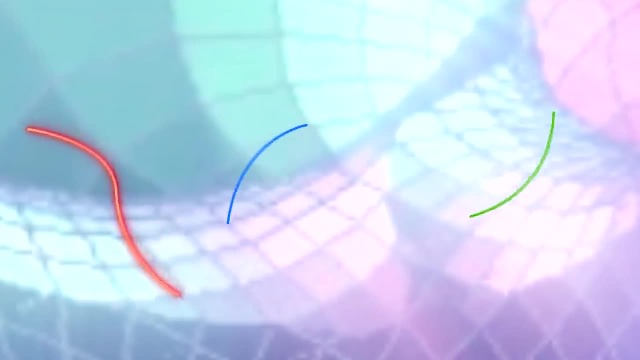 and specific dimensions could account for different color charges of the quarks- red, blue and green. So, for example, we could have two up quarks of different colors and one down quark of a third color. This would be a proton, since they are made up of two. 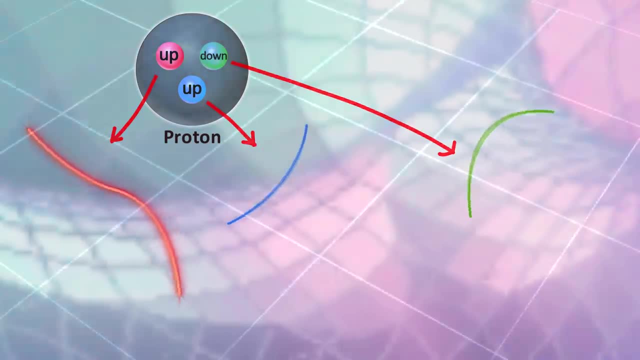 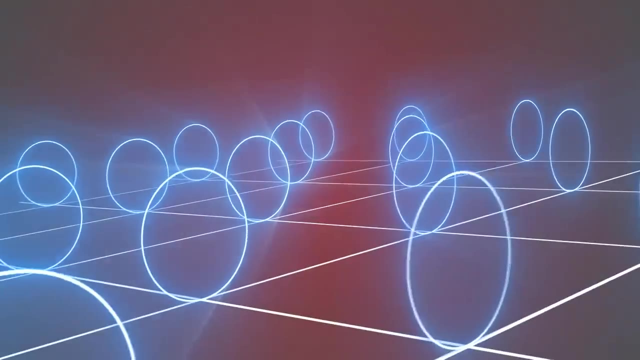 up quarks and one down quark. Note that the 6 dimensional Calabi-Yaw manifold depicted here as a 3D like structure is for illustration purposes only. The six small spatial dimensions are not something that we can imagine with our three dimensional minds. The actual structure: 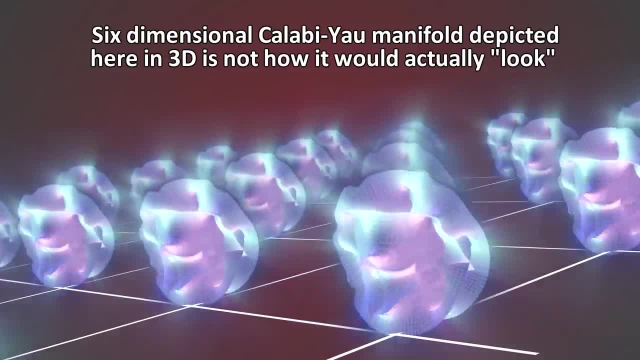 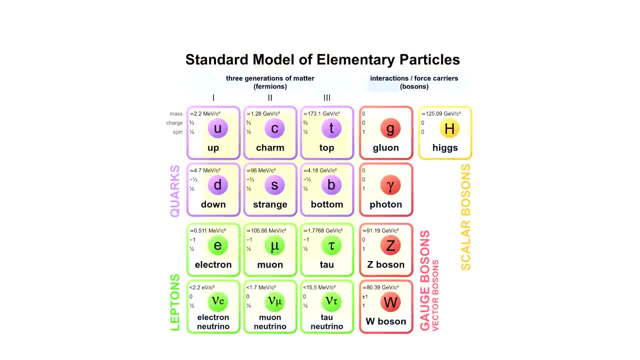 of this manifold and the vibrations within it is not something that can be visualized, particularly if you add the dimension of time to this picture. The promise of string theory is that most, if not all, of the fundamental constants could come out of it. In addition. 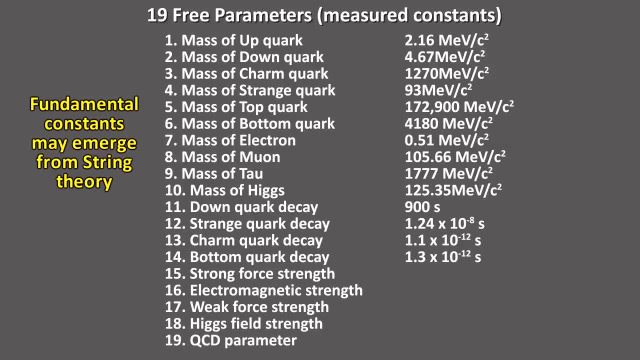 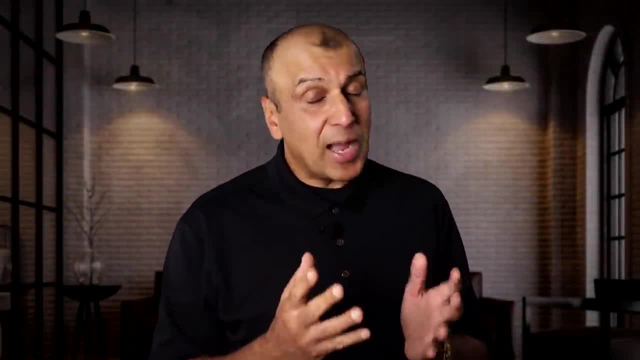 all the charges and properties of fundamental particles could emerge. This would be huge. It would be a true theory of everything. It's ambitious, but it also has some problems, The most obvious of which is the idea of nine spatial dimensions. Some scientists 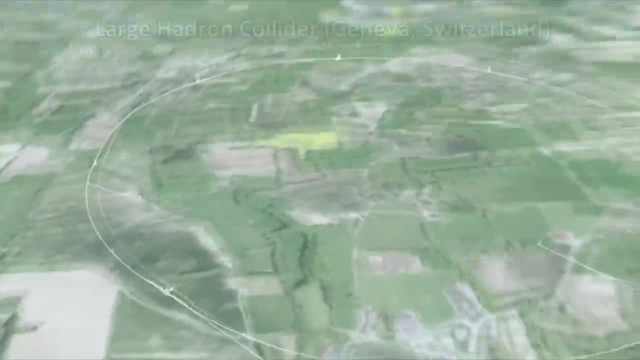 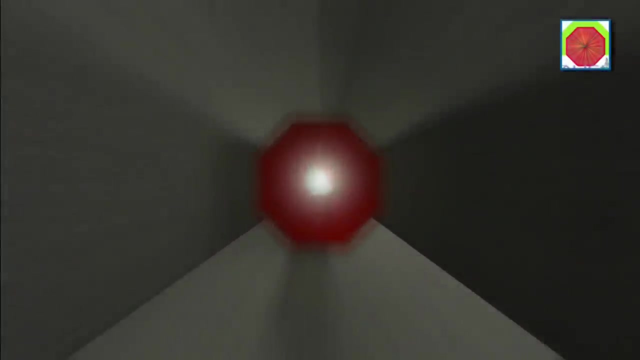 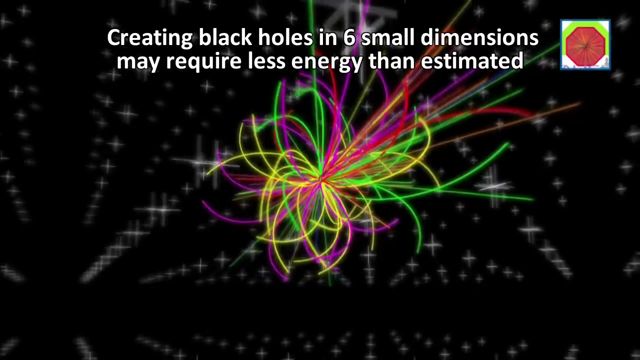 have attempted to detect this, for example, by creating microscopic black holes at the Large Hadron Collider, The idea being that if gravity is being diluted due to nine spatial dimensions, then creating black holes on very tiny scales in only the smaller six dimensions may require a lot less energy than in the same six plus our three larger dimensions. 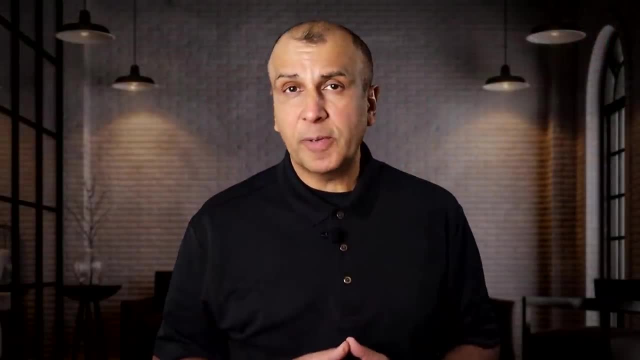 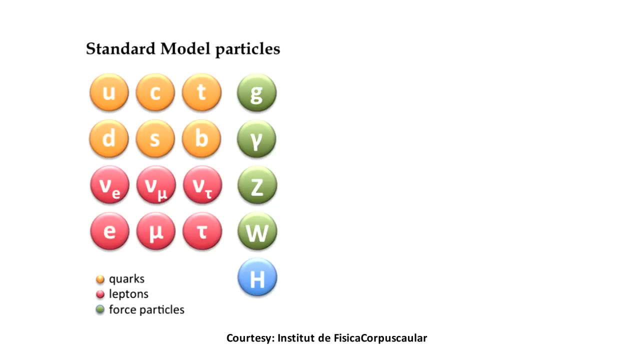 But so far none of this is true. No small dimensions have been detected in this or other experiments. The other problem is that superstring theory requires the existence of supersymmetry. This is the idea that each particle of the standard model has a shadow partner particle with different. 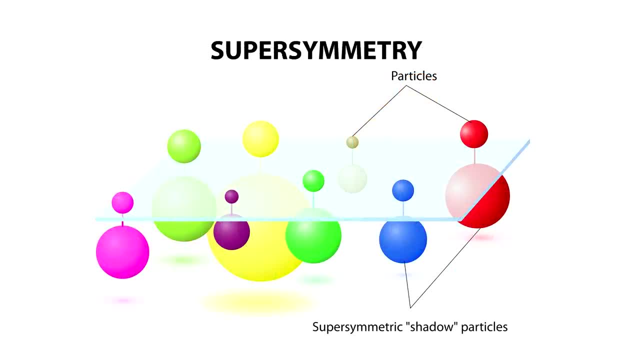 masses. The problem is that in a decade of searching for them at the Large Hadron Collider, no trace of supersymmetric particles has been found. String theory probably won't work without it. The reason that quantum gravity is such a difficult problem to solve is partly 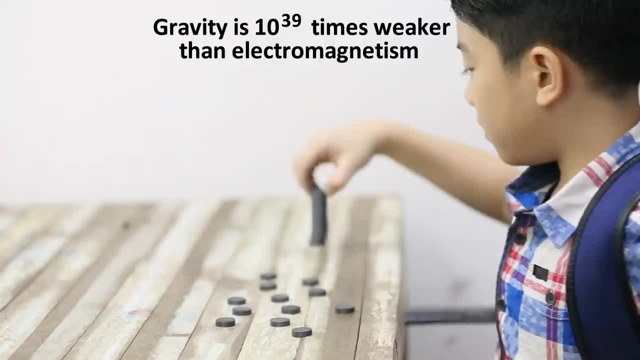 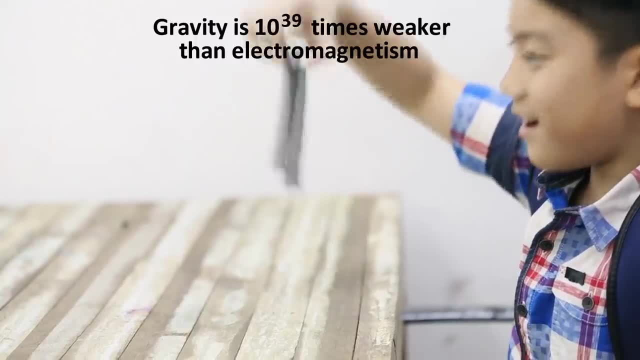 because gravity is so incredibly weak. For example, it is ten to the thirty-nine times weaker than electromagnetism. This is why a magnet can easily pick up another magnet against the pull of the entire Earth. We may never be able to detect the effect of gravity. 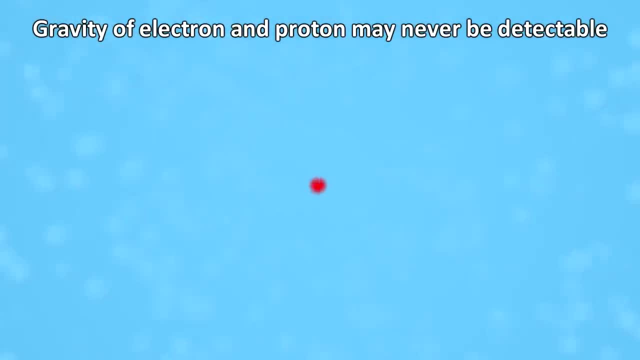 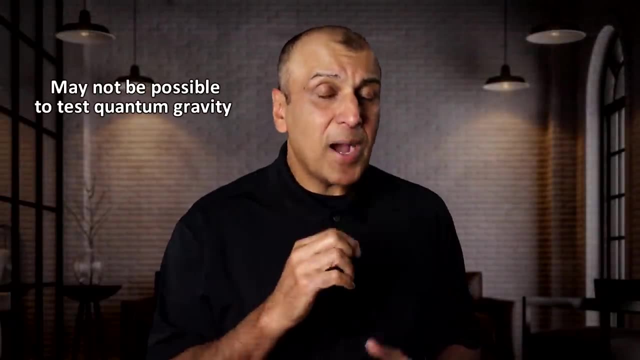 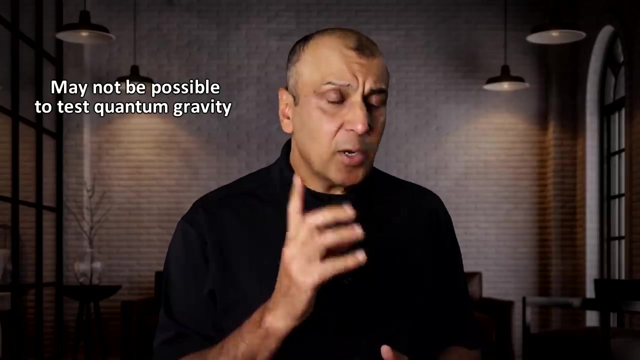 for example between an electron and a proton inside a hydrogen atom, It will be completely overwhelmed with the electromagnetic force between them. Quantum gravity predictions may be impossible to test. We may likely have to verify the theory through other predictions that such a theory makes Any theoretical formulation. 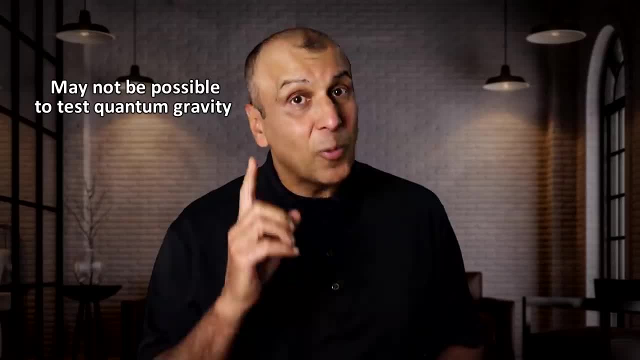 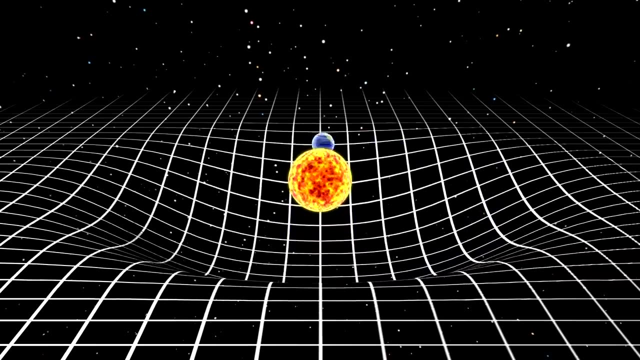 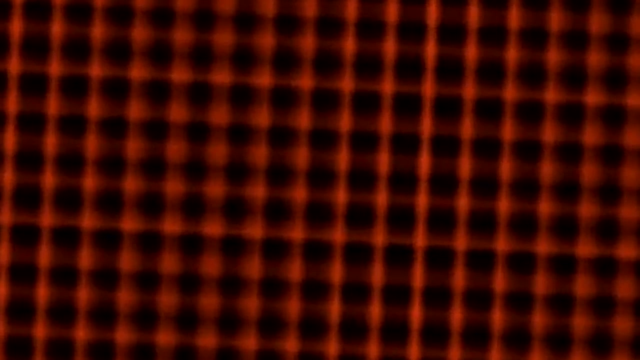 is almost certainly going to be driven by thought experiments rather than real experiments. Loop quantum gravity is inspired by Einstein's idea of treating gravity not as a force but as the curvature of the background. It just quantizes this background, But it largely ignores the other forces. This is why it's not currently a theory of everything, but a 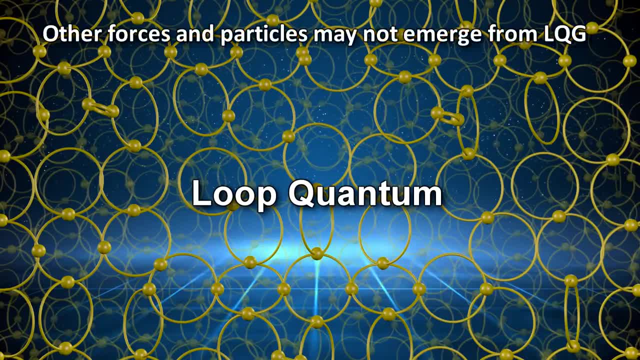 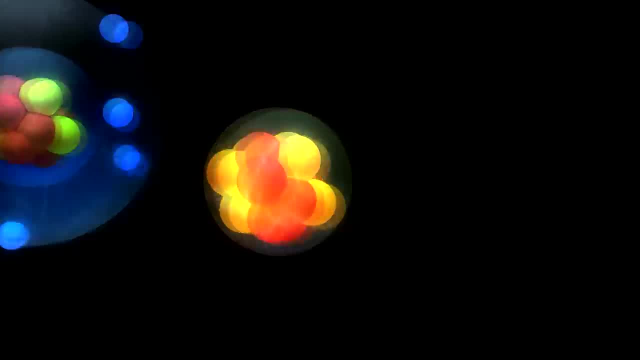 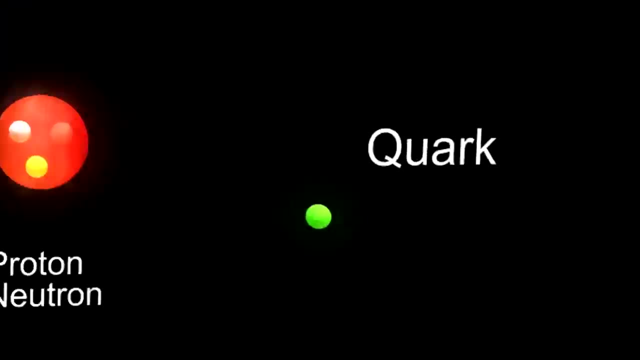 theory of quantum gravity clear that it can incorporate the other forces or particles of the standard model. On the other hand, string theory is inspired by the standard model but introduces a completely new mathematical formulation which attempts to bring gravity, along with everything else, into the fold. But it assumes that space and 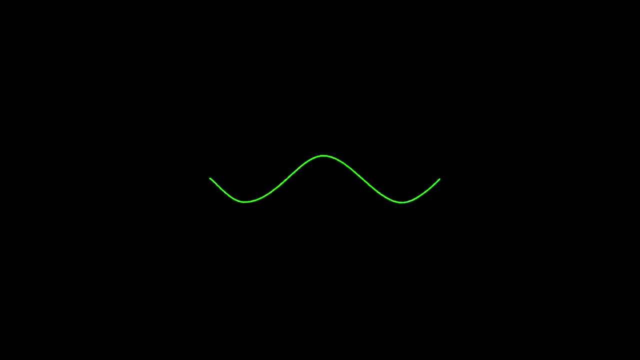 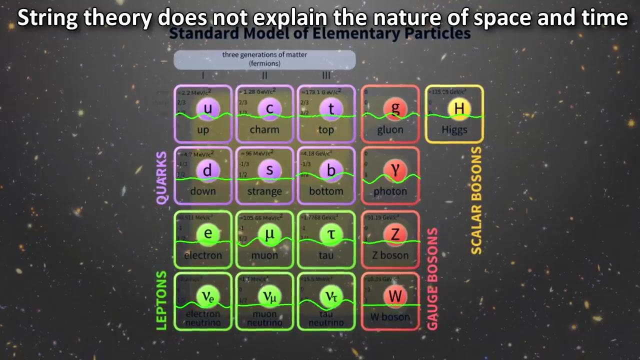 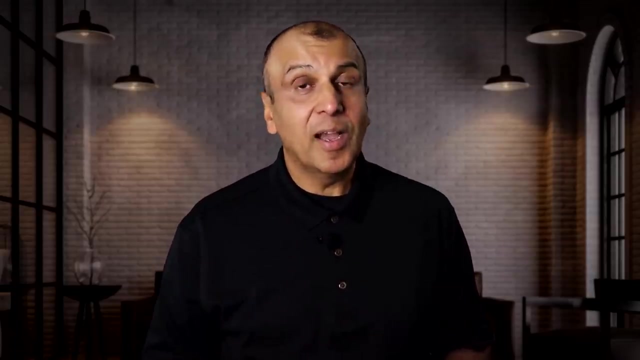 time already exists and does not attempt to create them. So in that sense the nature of the background, the space and time, is not something the string theory can answer. So neither theory at this point is well developed enough to be a satisfying theory of quantum gravity, let alone an all-encompassing theory of. 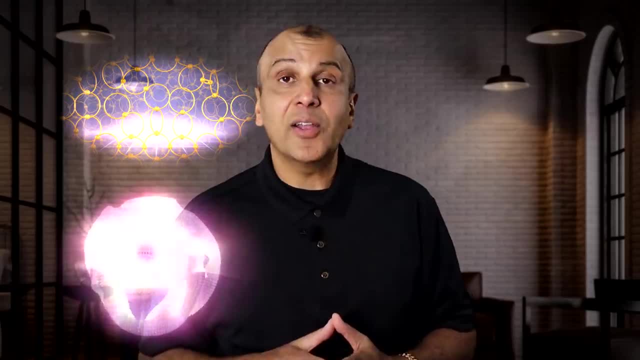 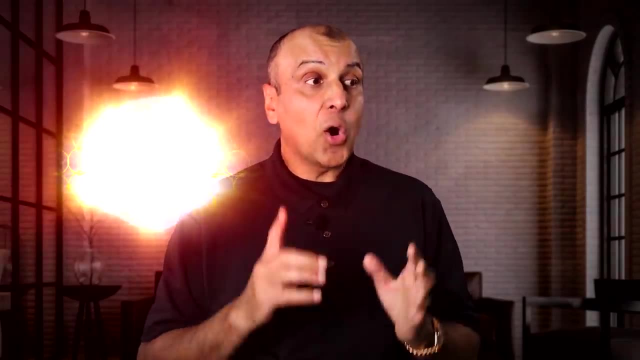 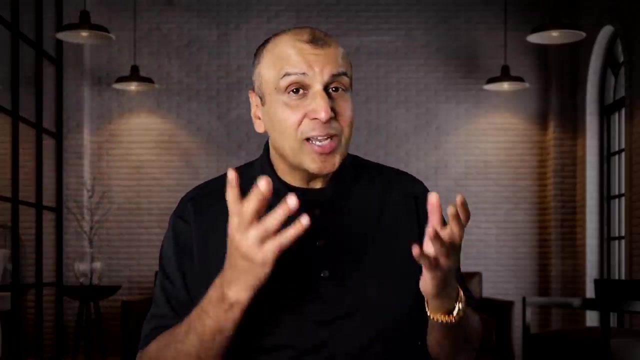 everything. Now what if these two theories could be combined together? That could be exciting, and some researchers are working on this very idea, So that could be the next big thing. Or, of course, all this could be wrong, But we won't know that until the next Einstein comes along and shows us mortals how the